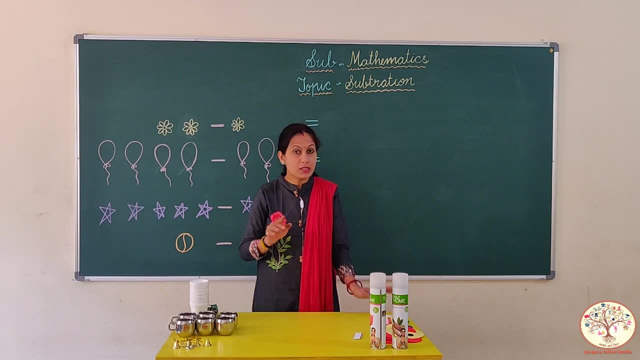 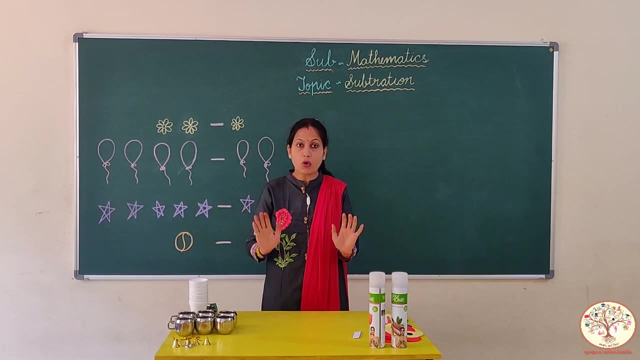 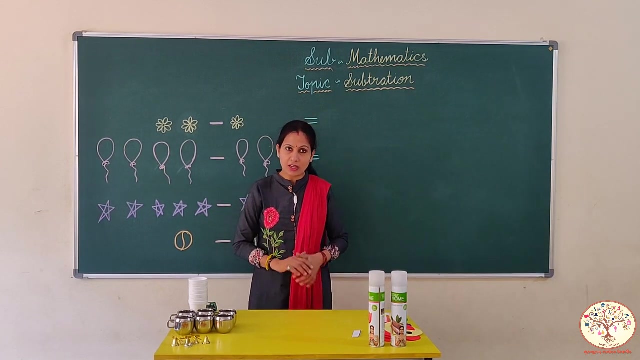 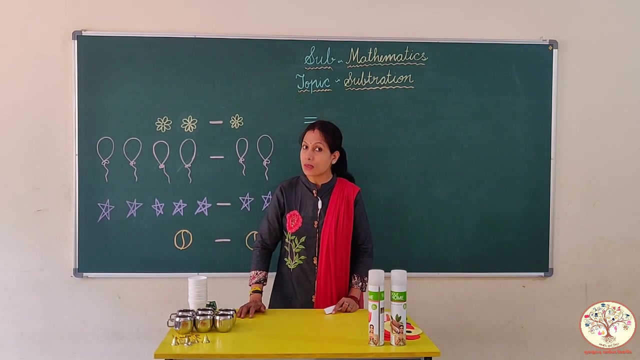 What is subtraction? Subtraction means taking away, to remove. After subtracting these objects, how many remaining, how many left know this? So, kids, today we will do addition with the help of some objects. Can you see them, Okay? and then we will do. 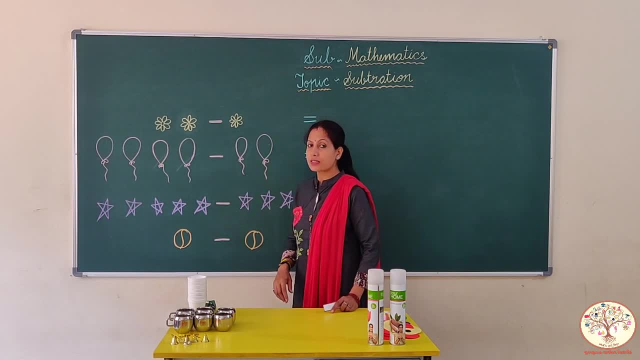 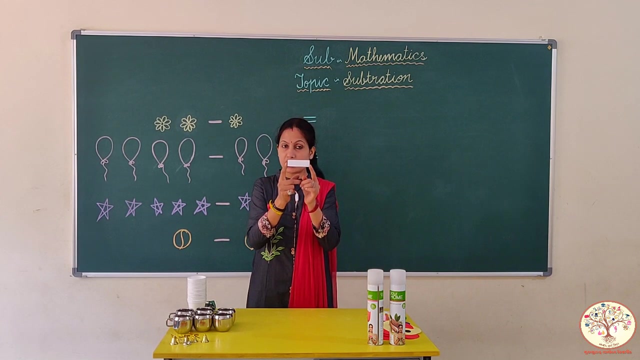 We will do subtraction with the help of these pictures. First. you look here. What is this? This is the symbol of subtraction. We say it: minus sign, Okay. what is this Symbol of subtraction? minus sign, Okay. so, kids, let us start. Look here. 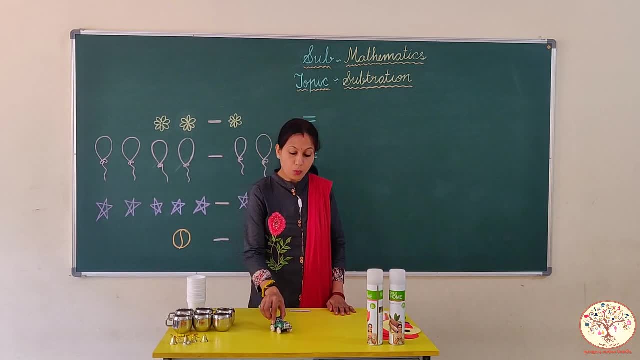 I have one card, Okay, and I drive it and take it away. One card was with me and I drove it and took it away. Now, how many cards are there? No card: If you have only one thing and that one thing goes away, then we have nothing. 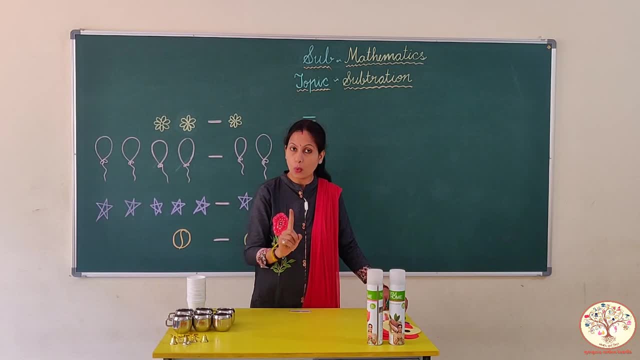 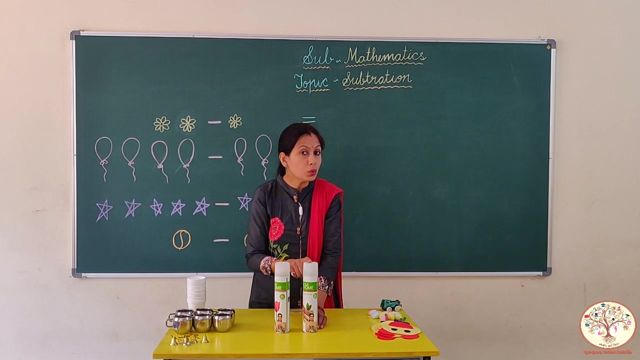 Nothing. That means zero. One minus one is equal to zero. Okay, now look here I have two room fresheners. Let us count them One, two. How many room fresheners are there? Two room fresheners, One, two. 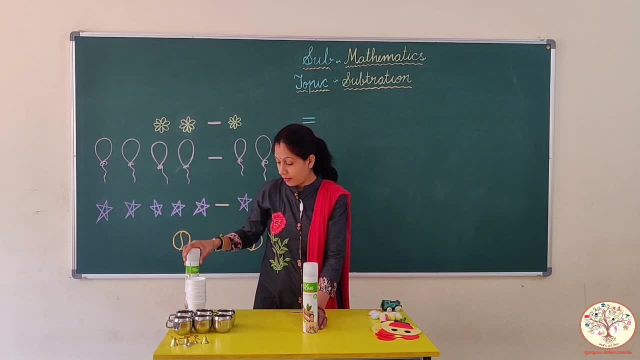 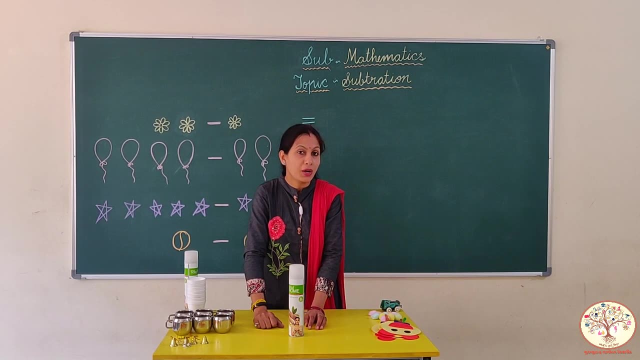 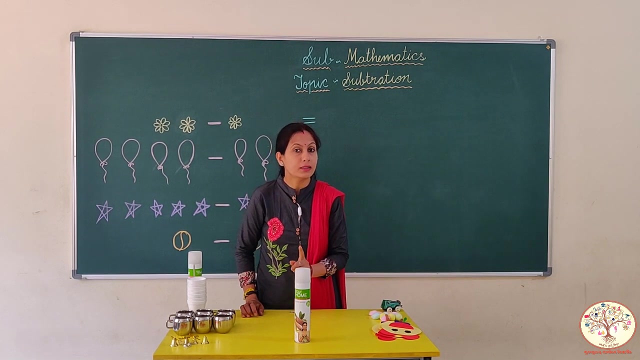 Now, if I take away one room freshener, How many room fresheners are left? Now I have only one. There is only one room freshener. So two minus one is equal one. Two minus one is equal one. Okay, now, kids, I have some bells. 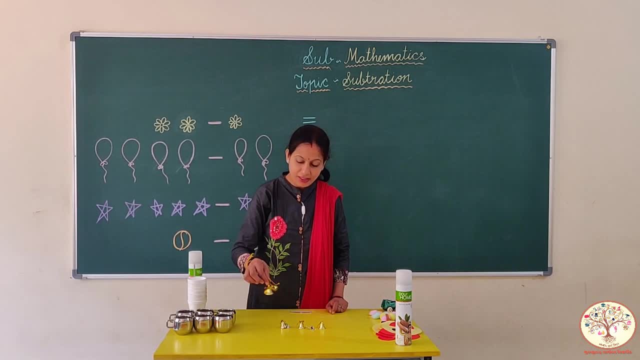 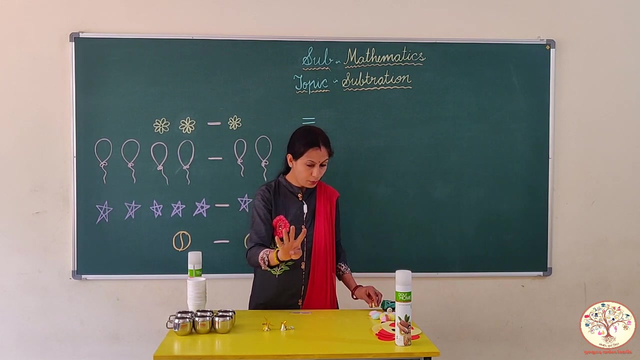 Look here Bells. Let us count them: One, two, three, four. How many bells are there? Four bells: One, two, three, four. Now if I take away two bells, One, two, Now how many bells I have? 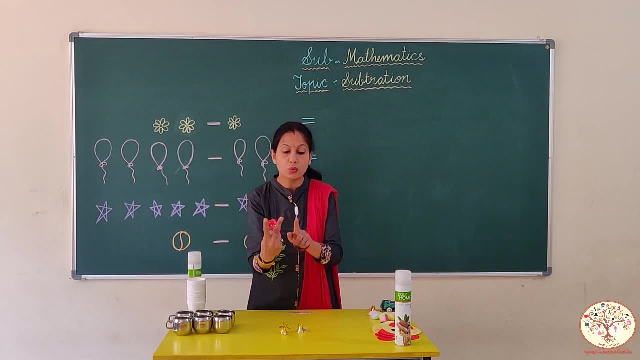 Two bells Now: one, two, One, two. Two bells are left. Okay, kids, look here, I have some Teddy Faces. Let us count them. One, two, three, four, five. One, two, three, four, five. 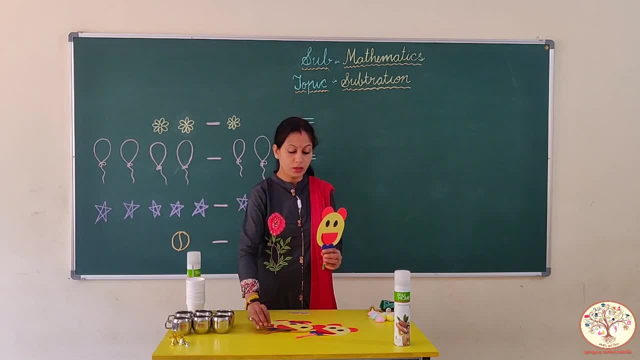 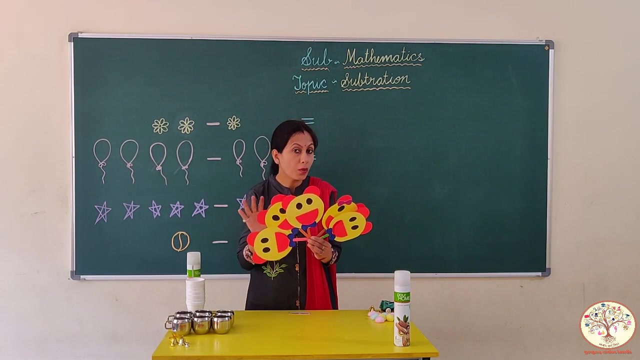 Now, how many bells are there? Two, two, three, four, five. Two, two, three, four, five. Two, two, three, four, five. I have 5 sturdy faces Now, if I remove 3 faces from here, 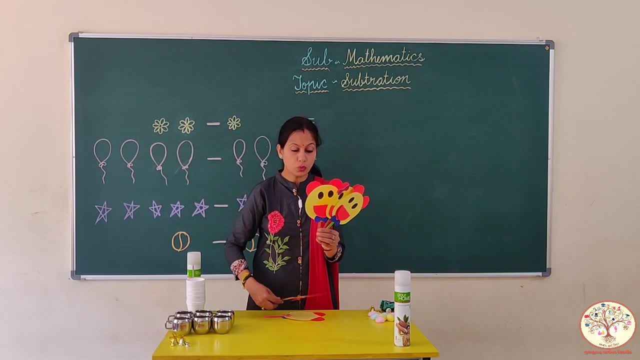 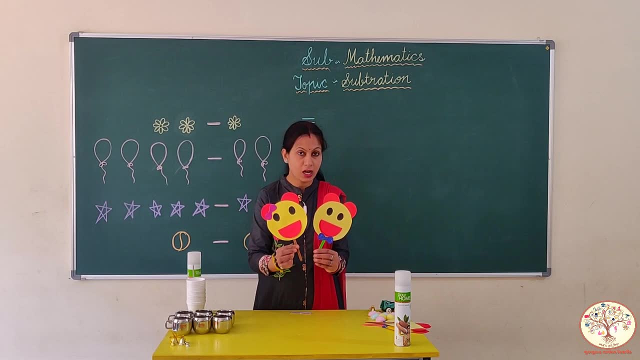 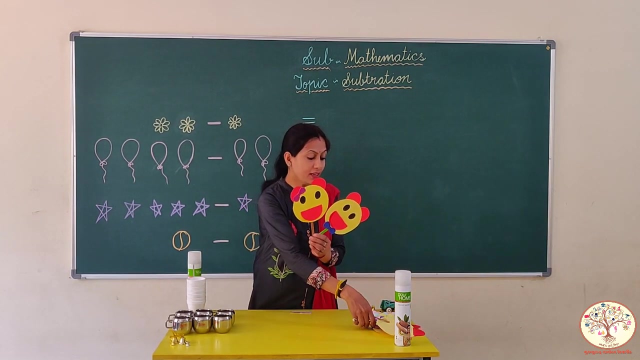 1, 2 and 3.. How many faces are left? Let's count 1, 2.. Now there are only 2 faces, So 5 minus 2.. Sorry, 5 minus 3 is equal to 2.. 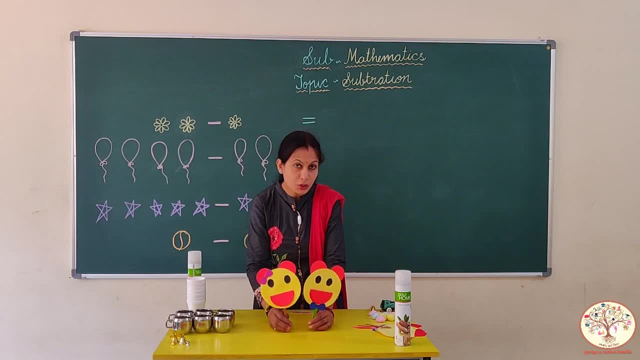 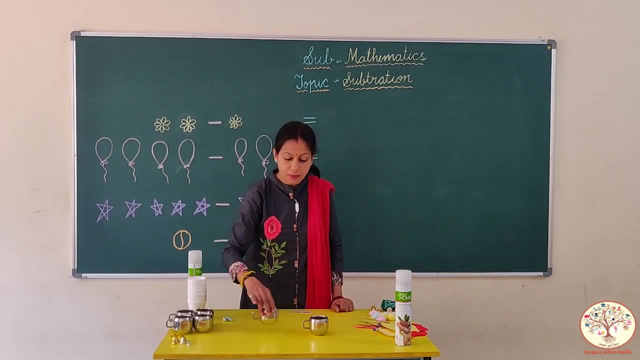 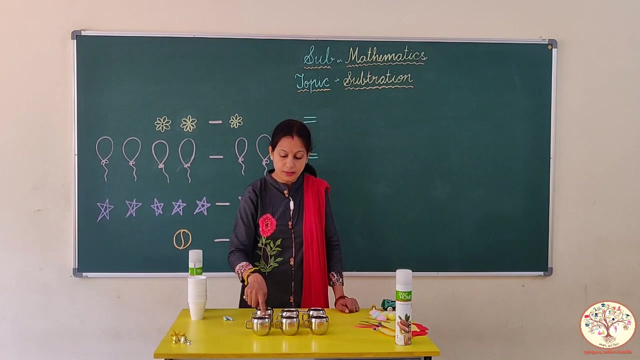 If 3 is minus from 5, then we have 2 teddy faces left. Okay, Now kids, look here, I have some cups. Let's count 1,, 2,, 3,, 4,, 5,, 6.. 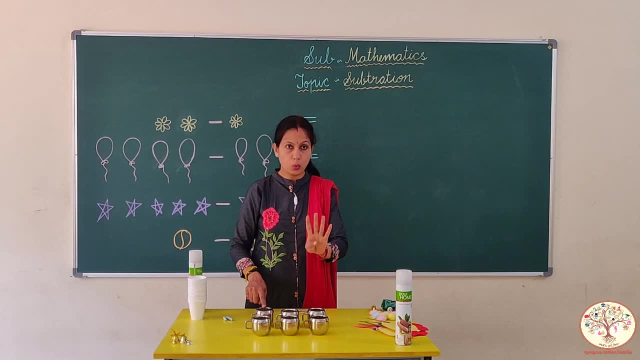 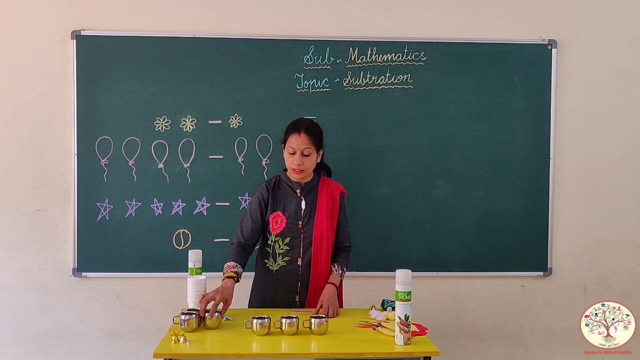 1, 2,, 3,, 4,, 5, 6.. If I take away 3 cups- 1,, 2, 3.. 1,, 2, 3. How many cups are left? Tell me? 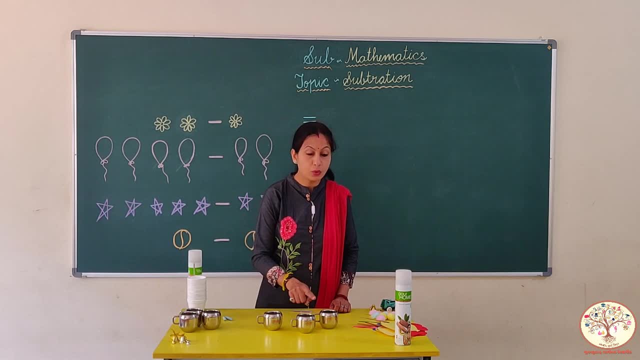 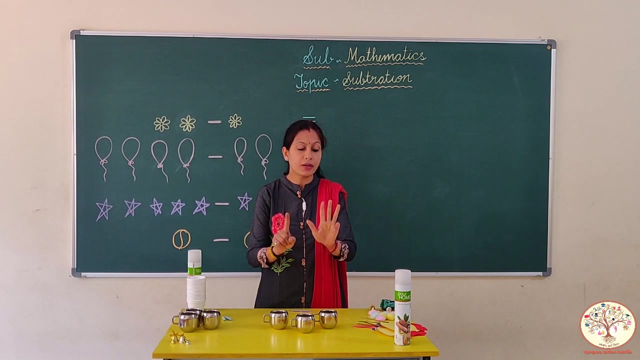 Let's count them Okay: 1,, 2,, 3.. Now there are only 3 cups left: 1,, 2,, 3,, 4, 5, 6.. Minus 3. 1,, 2, 3.. 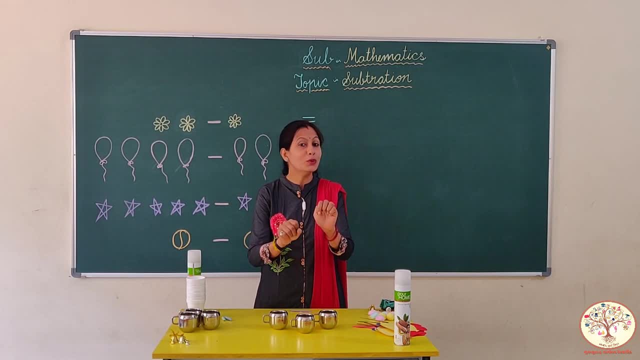 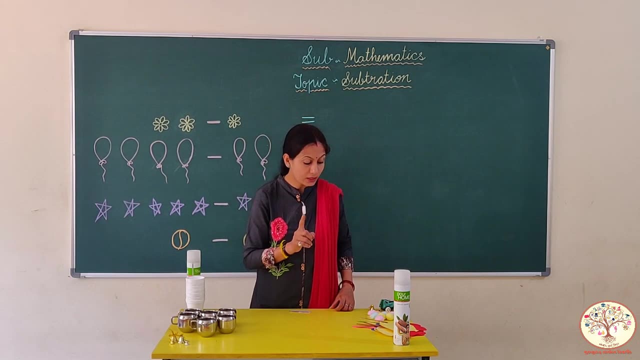 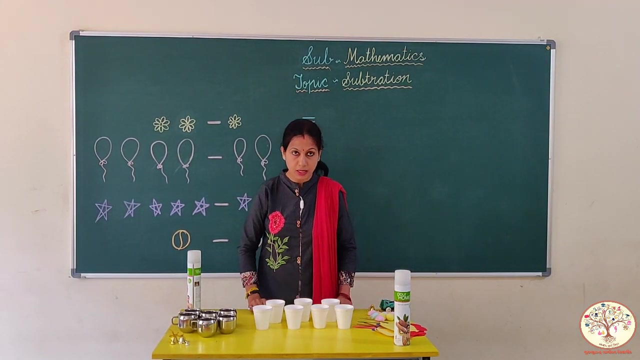 How many left? 1,, 2,, 3.. Okay, 6 minus 3 is equal 3,. okay. Now, kids, I have some disposal glasses, Glasses 1,, 2,, 3,, 4,, 5,, 6,, 7.. 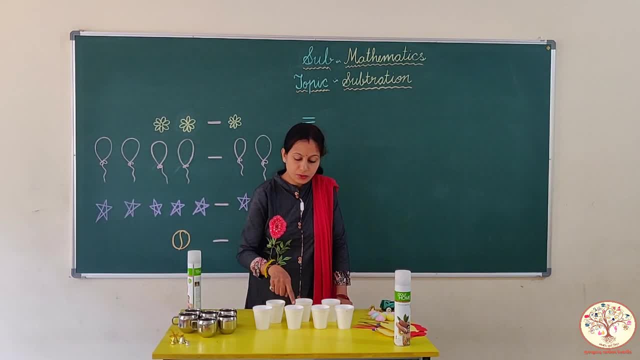 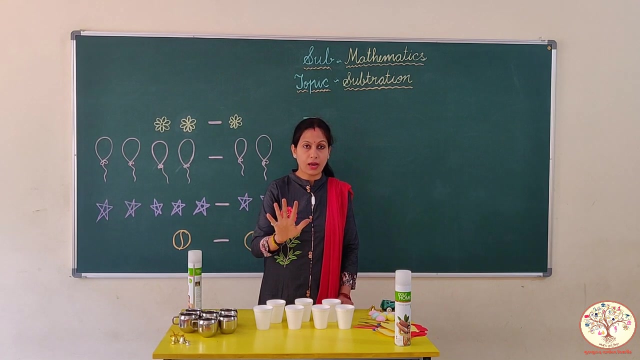 Let's count once again: 1,, 2,, 3,, 4,, 5,, 6, 7.. I have 7 disposal glasses: 1,, 2,, 3,, 4,, 5,, 6, 7.. 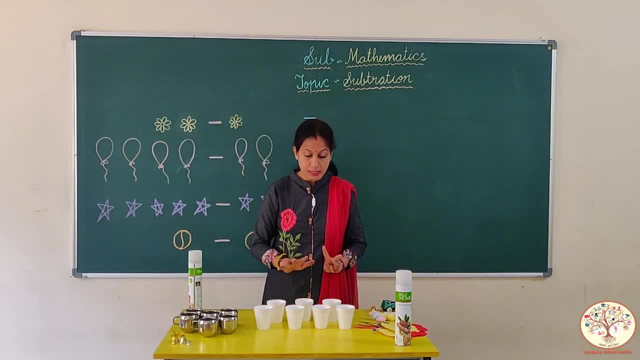 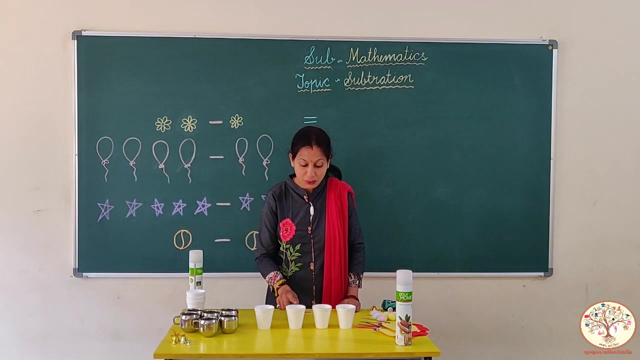 If I take away 3 glasses from here? 1,, 2, 3.. How many glasses are left now? Tell me? let's count, Okay: 1, 2.. 1,, 2,, 3, 4.. 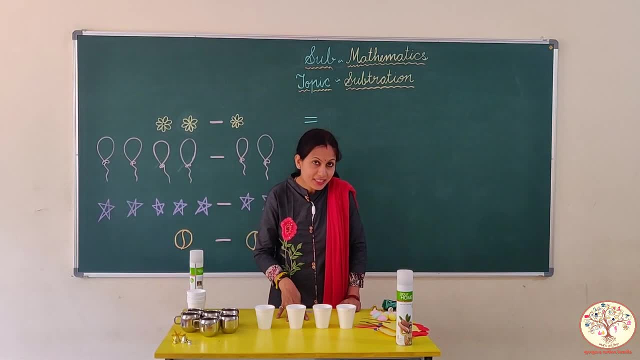 Now 4 glasses left here: 1,, 2,, 3,, 4,, 5,, 6, 7.. Minus 3.. 1, 2, 3.. How many left? 1,, 2,, 3,, 4.. 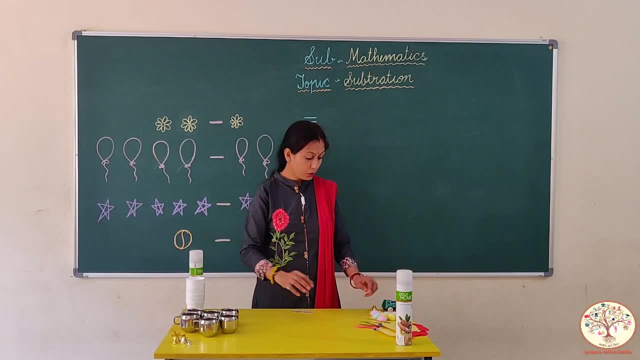 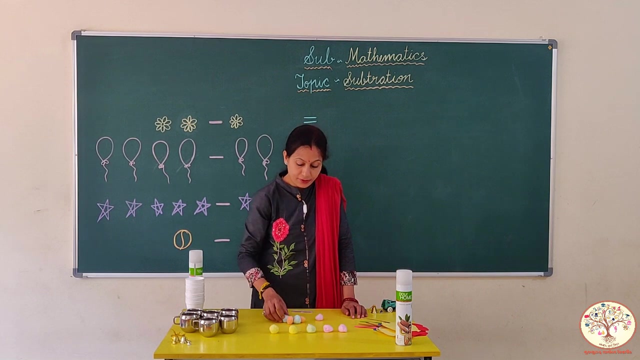 4 glasses. Now look here, What do I have? These are pom-poms. Let's count them: 1, 2, 3, 4,, 5,, 6,, 7,, 8,, 9,, 10.. 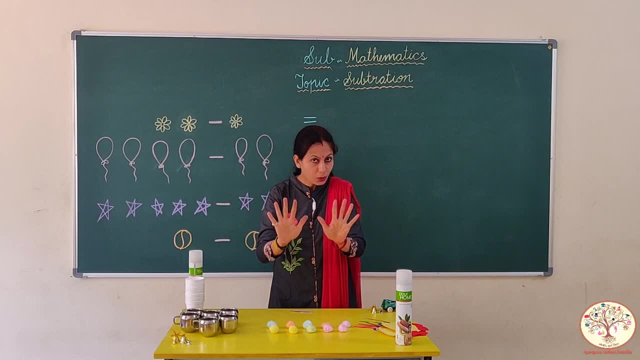 I have 10 pom-poms, Okay: 1,, 2,, 3,, 4,, 5,, 6,, 7,, 8,, 9, 10.. 10 pom-poms If I take away 5 pom-poms. 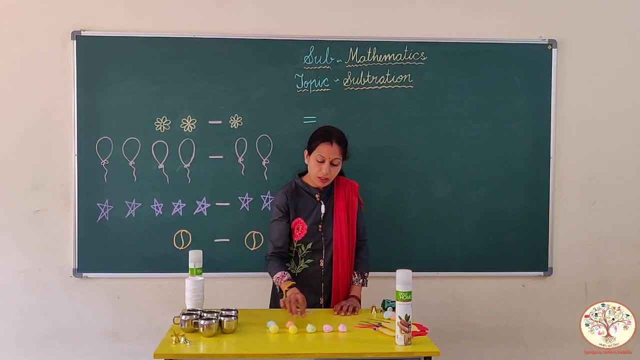 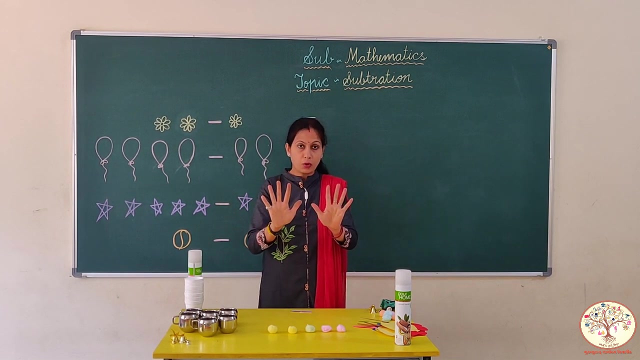 1,, 2,, 3,, 4, 5.. How many pom-poms are remaining? Let's count them: 1,, 2,, 3,, 4, 5.. From 10, we minus 5 pom-poms. 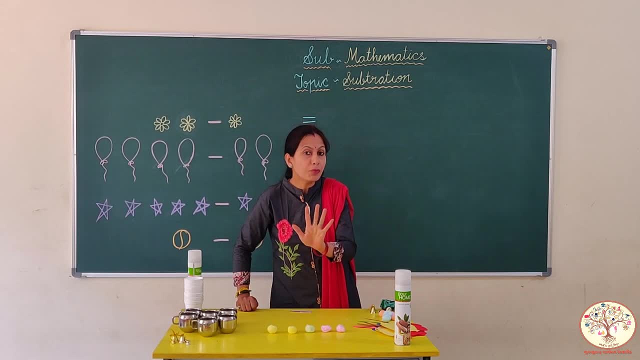 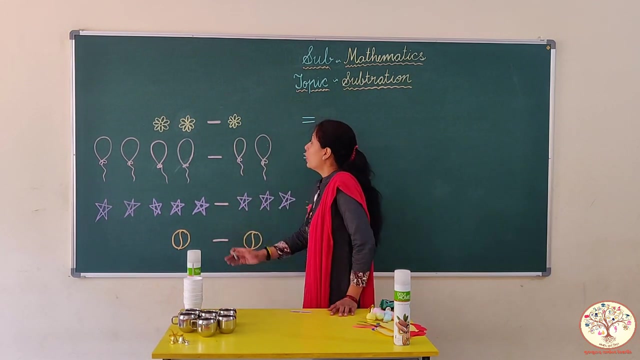 How many pom-poms are left? 5 pom-poms, Okay. So, kids, this is subtraction. Now we will do subtraction with the help of these pictures. Okay, So let's start. Look here. What are these? These are flowers. 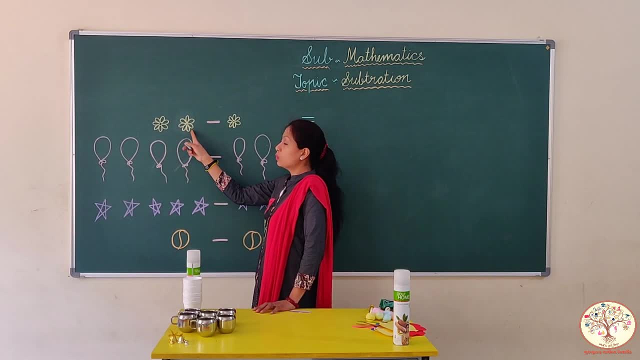 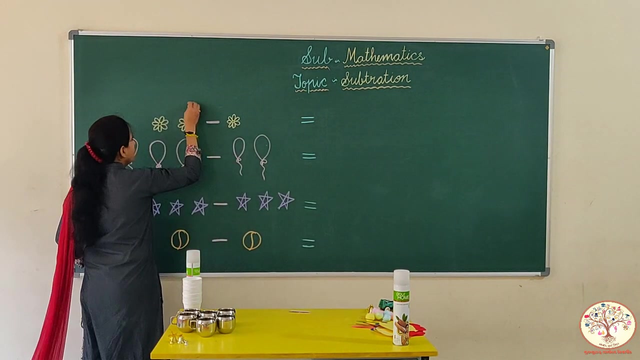 How many flowers? 1, 2.. 2 flowers, 2 flowers. This is the symbol of minus Minus 1 flower. 2 flower minus 1 flower. 2 minus 1. Is equal if I take away 1 flower. 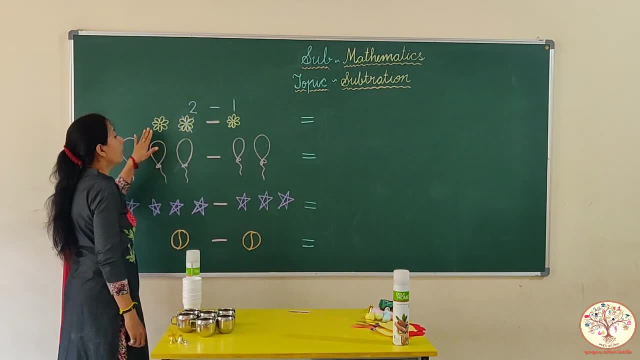 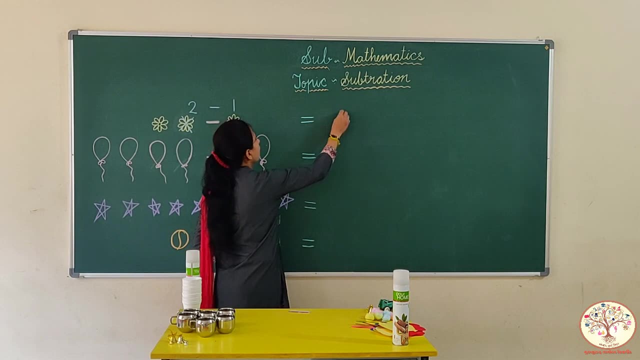 How many flowers are left? Only 1 flower, So 2 minus 1,. this is the symbol of equal to Equal to 1 flower, So 2 minus 1.. This is the symbol of equal to Equal to 1 flower. 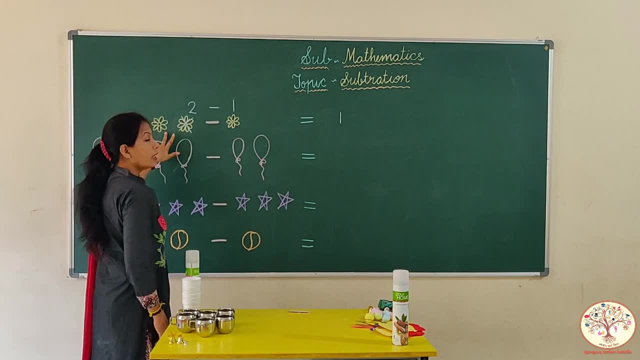 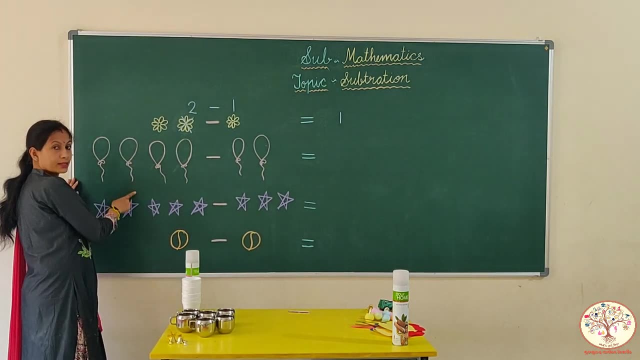 2 flowers. If we take away 1 flower from 2 flowers, then we will have only 1 flower. Now look at these. What are these Balloons? Do you like balloons? Yes, Let's count them: 1,, 2,, 3, 4.. 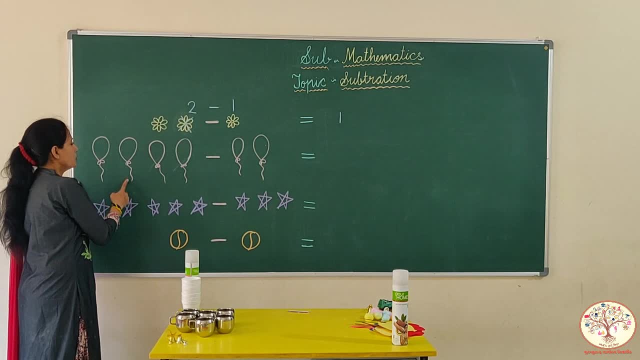 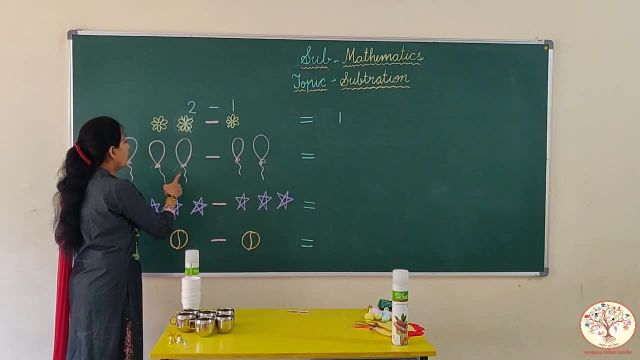 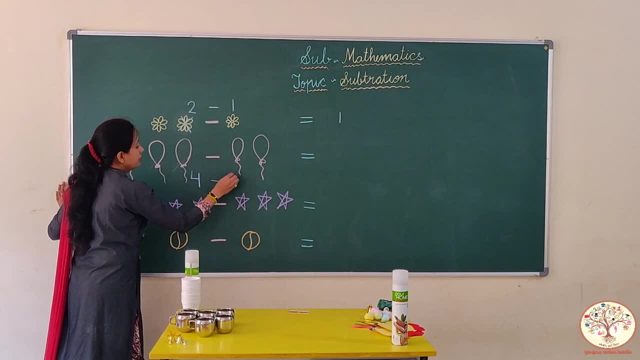 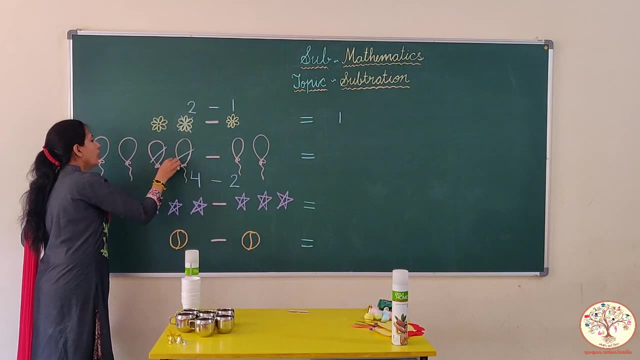 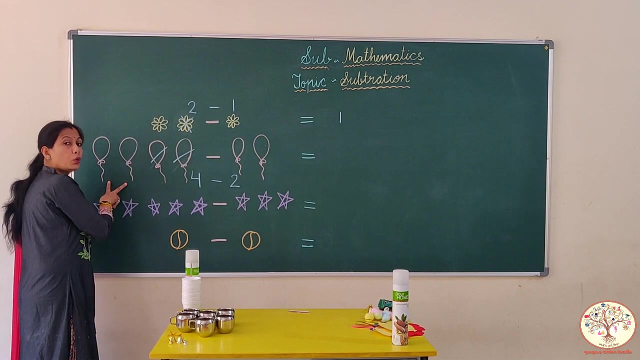 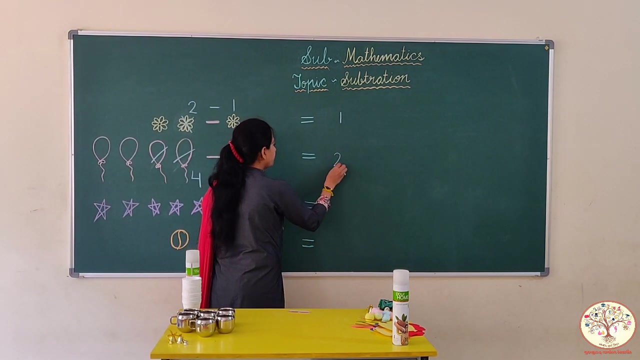 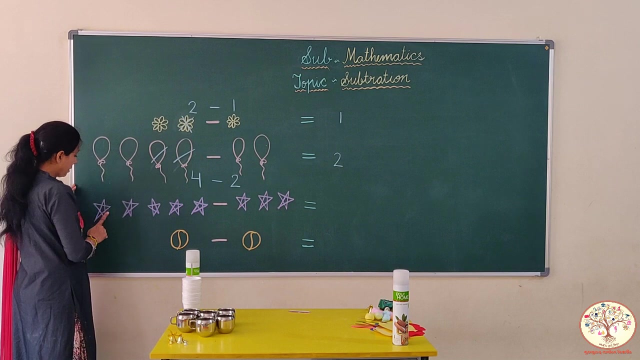 은 2, 2 balloons. If we take away 2 of 4 balloons, we are left with 2 balloons: balloons 1, 2.. 4 minus 2 is equal to 2.. Okay, Now look at these pictures. These are stars. 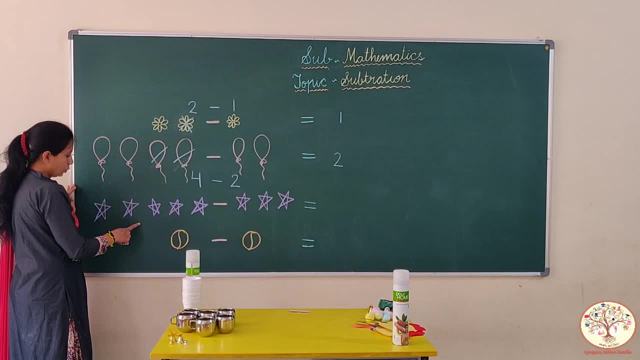 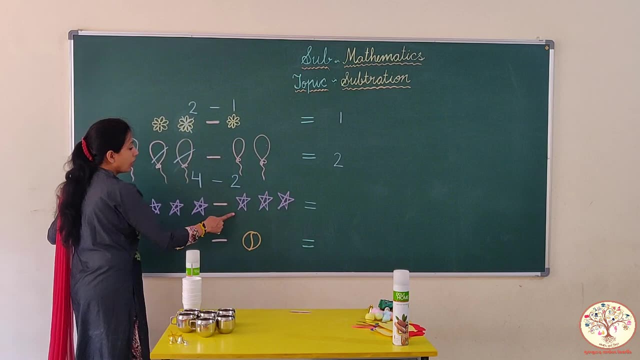 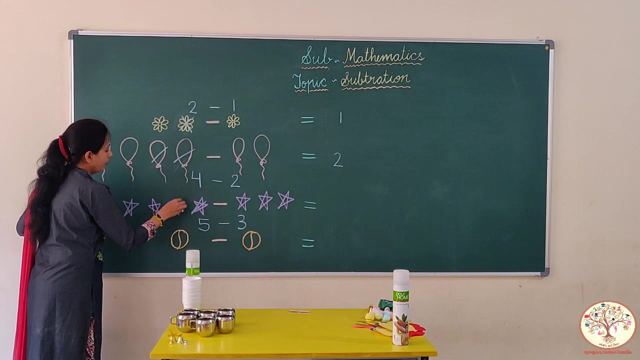 Let's count them: 1,, 2,, 3,, 4, 5.. 5 stars minus 1, 2, 3.. 3 stars, 5 stars. 5 stars minus 3 stars: Okay, I take away 3 stars from 5 stars. Okay, 1,, 2, 3.. Now I left with 1, 2.. Only 2 stars. 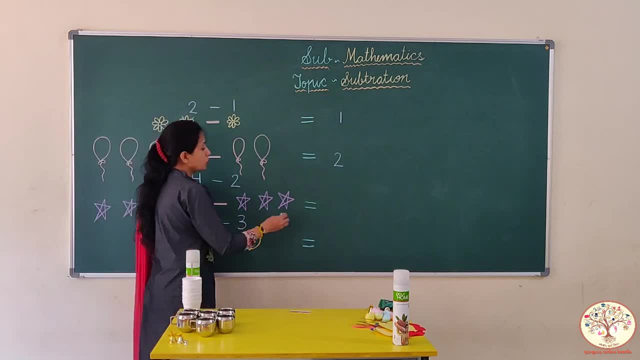 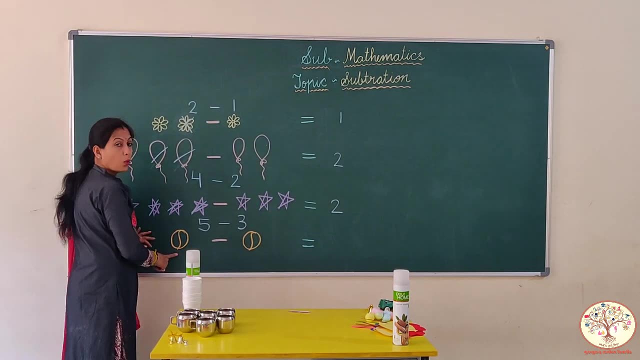 5 minus 3 is equal to 2.. Okay Now, kids, there is 1. Minus 1 ball. Minus 1 ball: 1 minus 1.. As we saw earlier, there was 1 car And 1 car went away. So we have no car, Nothing, 0.. 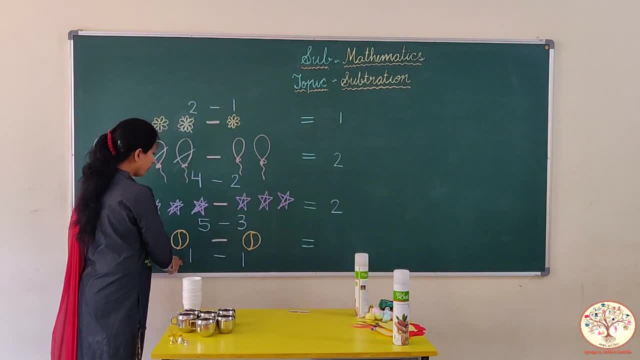 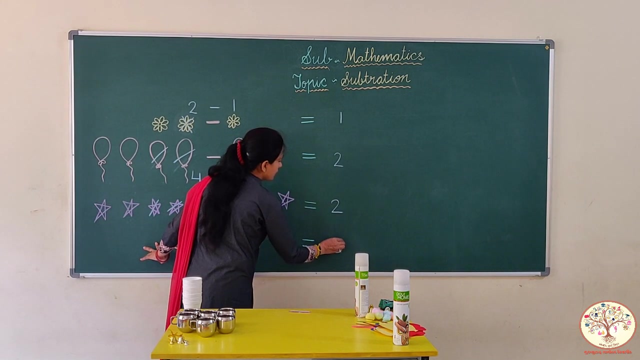 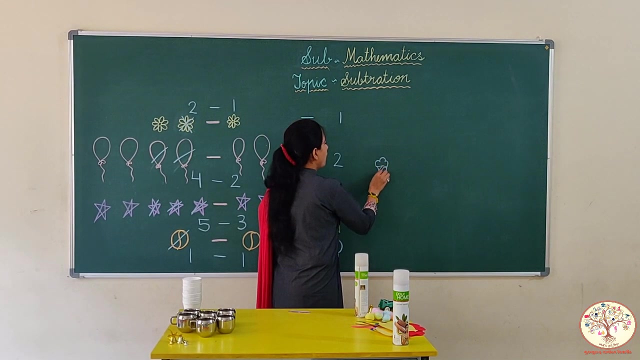 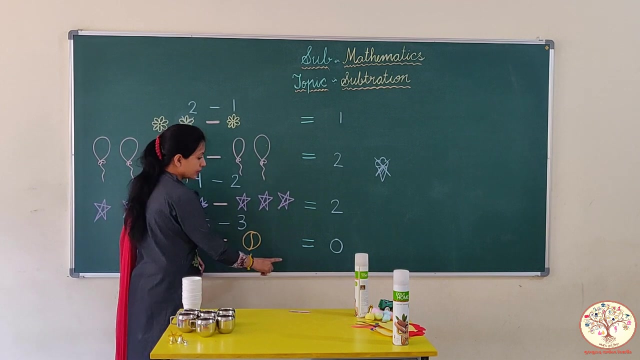 So 1 minus 1.. I take away 1 ball. Now I have no ball. 1 minus 1 is equal to 0.. You will have only one ice cream And you will eat it, So you will have ice cream after eating. You will not have 0 ice cream, Nothing. So 1 minus 1 is equal to 0.. 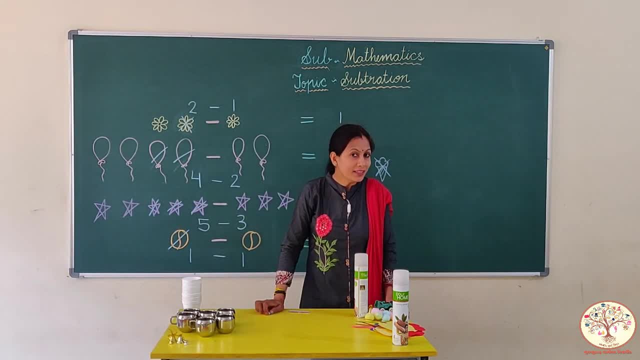 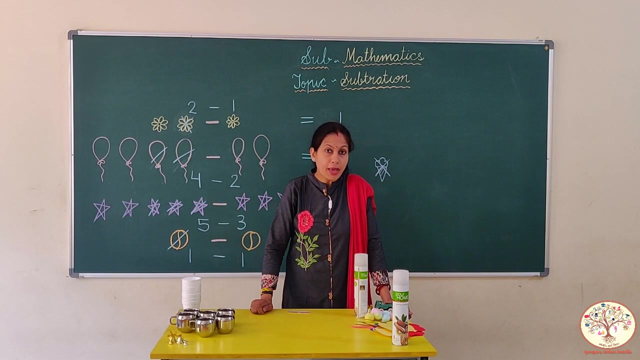 So, kids, today we learned subtraction. We learned with the help of some objects and with the help of some pictures. So do practice of subtraction at your home. We will come back with a new exercise of subtraction in our next video. Till then, stay tuned.